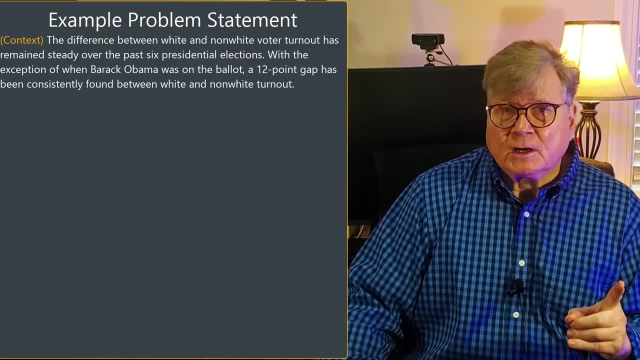 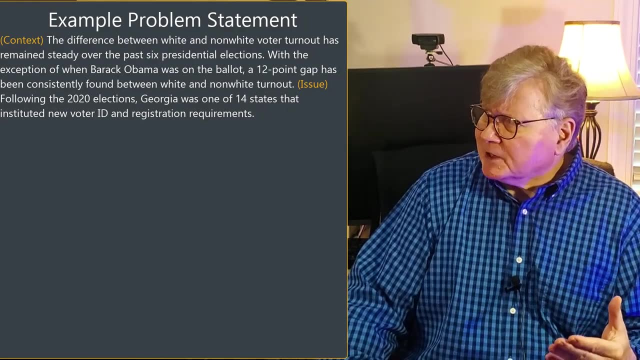 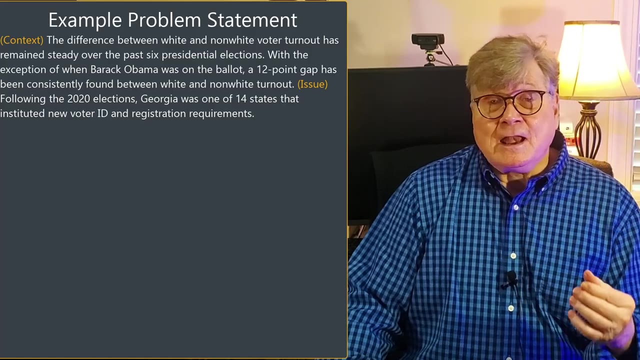 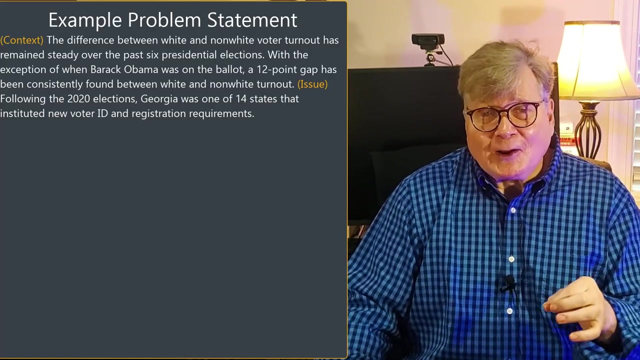 and non-white voter turnout. Next comes the issue Following the 2020 elections. Georgia was one of the most populous states in the United States- 14 states that instituted new voter ID and registration requirements, So now the issue has been narrowed to the new voter laws passed by the state of Georgia following the 2020 election. 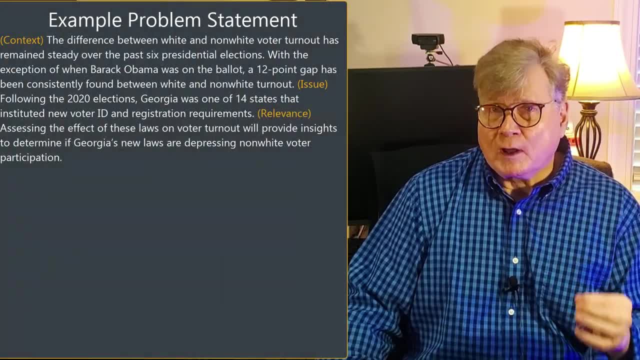 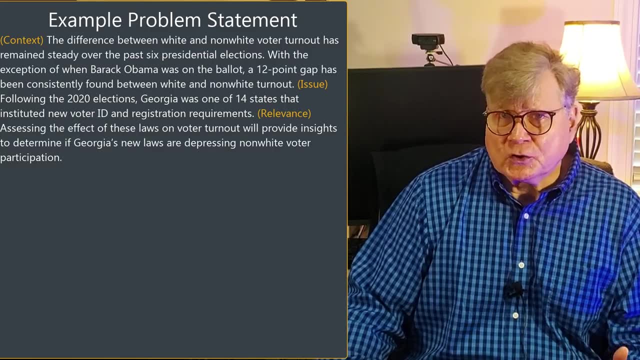 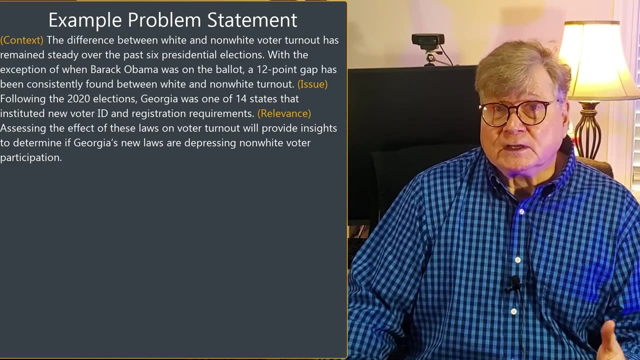 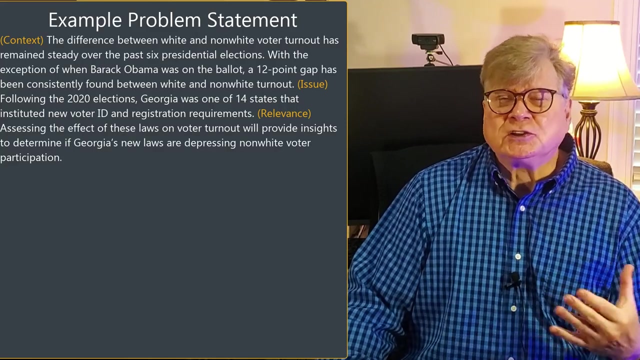 That's narrow. Next comes relevance, or why we should know about this. Assessing the effect of these laws on voter turnout will provide insights to determine if Georgia's new laws are depressing non-white participation in elections. In other words, this section provides the justification for doing the entire research project. 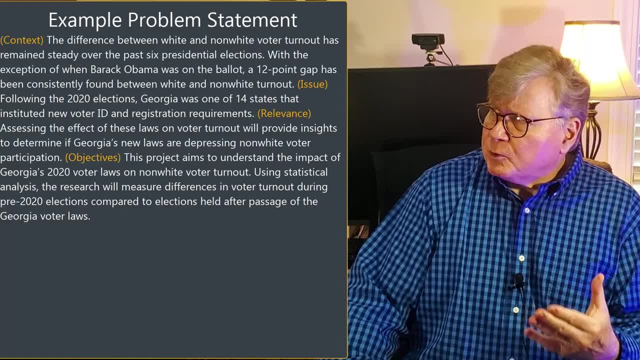 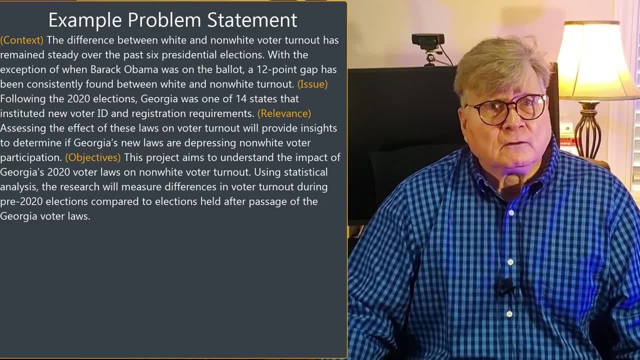 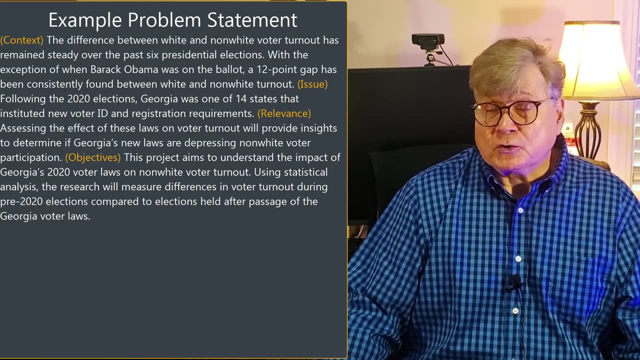 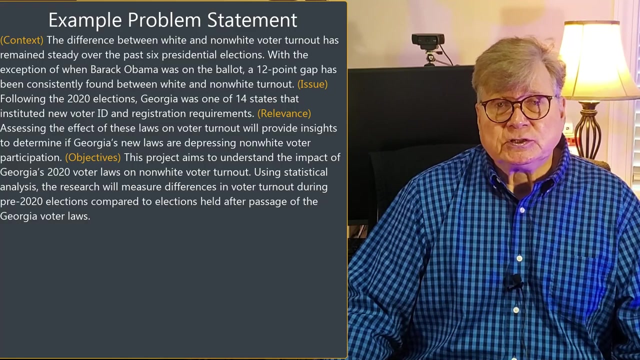 And, finally, are the objectives. This project aims to understand the impact of Georgia's 2020 voter laws on non-white participation in elections. Using statistical analysis, the research will measure differences in voter turnout during pre-2020 elections compared to elections held after passage of the Georgia voter laws. 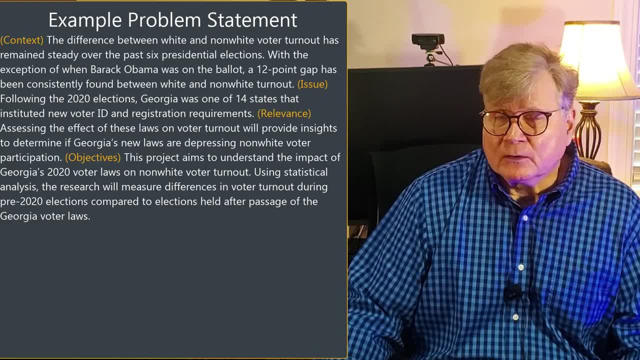 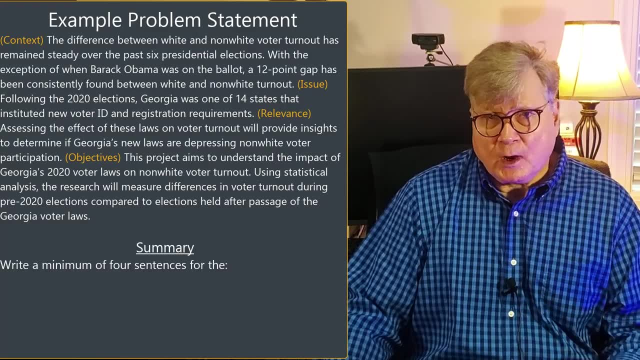 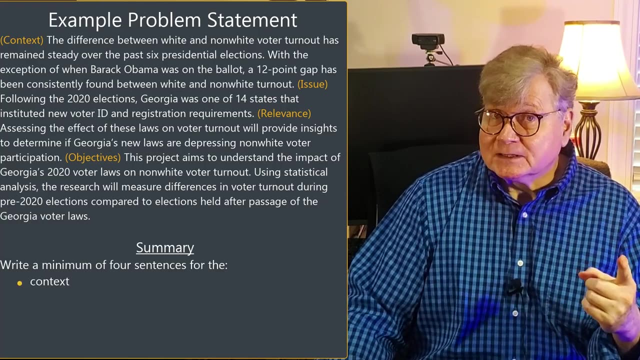 So, in other words, what has been the impact of these new laws? That's what you hope to find out. So, to sum up, for your problem statement, be sure to write a minimum of four sentences for the context issue: relevance and objectives. 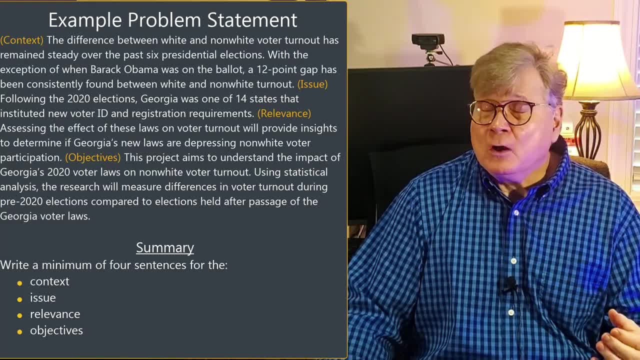 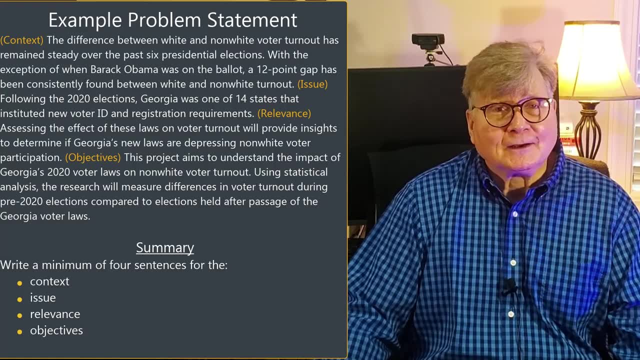 Now, naturally, you can add more sentences if you need to, but those are the four essential elements of any problem statement. Okay, good luck with your problem statement. 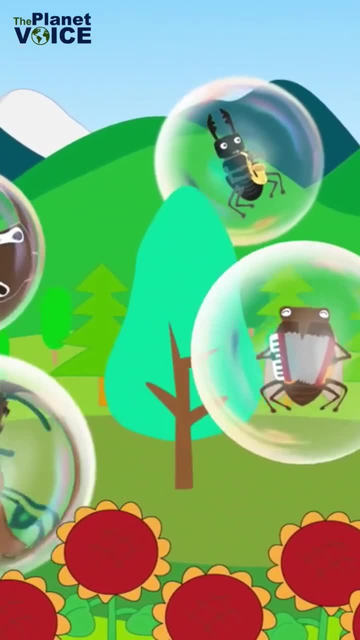 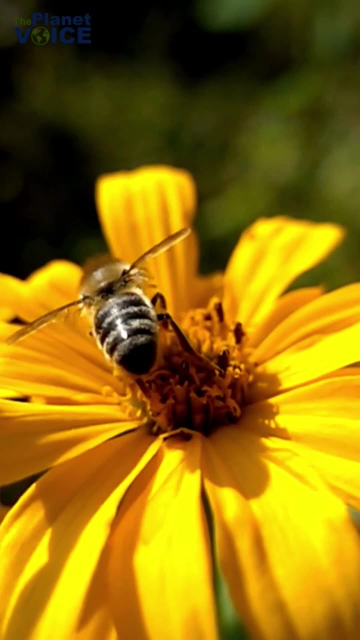 Insects play an essential role in the functioning of ecosystems and are critical to the survival of many other species. As pollinators, insects help to ensure the production of crops and the growth of plants, which in turn provides food and habitat for other animals Without insects,